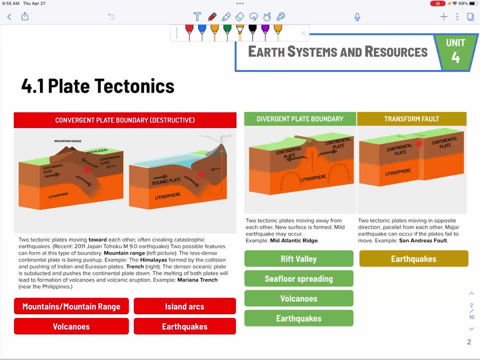 know them. So we have convergent plate boundaries and make sure you know the features that are listed down below, like the mountain ranges, island arcs, volcanoes and earthquakes- And the earthquakes are usually Very major- okay, Where we have for the places where we have divergent plate boundary, they are: 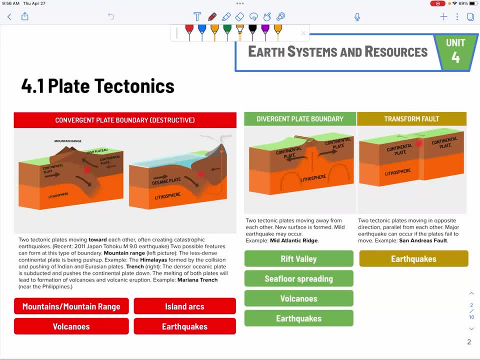 constructive. They create more land, more land surface areas, because the magma comes out and just cools off and then becomes just new land surfaces. We have a mid-Atlantic ridge as an example. So in the middle of the Atlantic Ocean, the Atlantic Ocean, we see the. 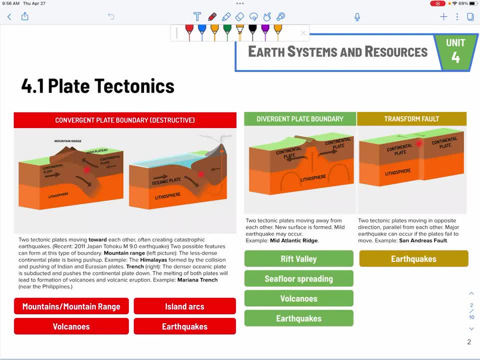 Projectiles are. usually We see the ocean spreading farther and farther away, So that's the main feature of the Atlantic Ocean. All right, We also see earthquakes, but they're not going to be very major compared to the ones that we see in the convergent plate boundary. And the last one will be Transform Fault and the. 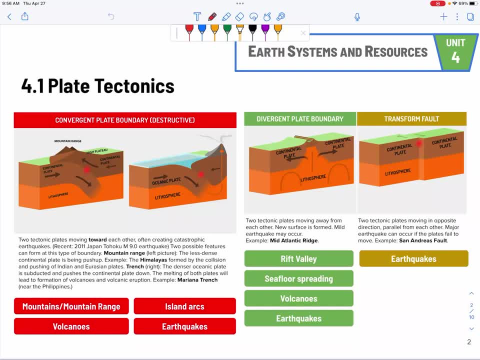 most famous one. it's going to be the San Andreas Fault in California, So earthquake will be the major one that we see. And then there are volcanoes, and we will see the polar bears there, and so we have one of the have power. Six dwarfs will be floating around drinks at a distance. so we have ourulative drivers and the blinkers, all the frozen Danshais and we can actually see. One person was all these small classmates that just left the hotel yesterday And, by the way, if you are a totslayers, there are so many of them in the area when you get around a night. 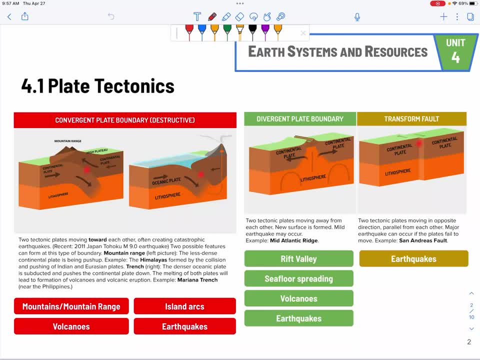 uh, and the earthquake could be pretty intense. now you may think about: wait, hold on, they're just moving parallel with each other. how would that be, uh, an intense, uh, earthquake? that's a very good point. and the thing it's uh, the plate boundaries, i mean the, i mean the two plates. 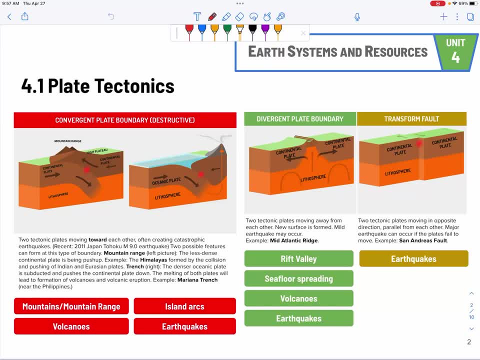 are not going to move pass each other in a perfectly parallel fashion. so, uh, so there will be some places where the pressures will build up and then that, when that pressure is being released, we will have a major, major earthquake. so, uh, if you live in the california or live somewhere, 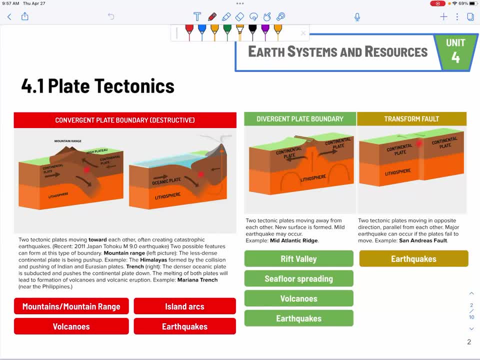 near the west coast. uh, you make online search about the big one that's, uh, that's already overdue as of 2023, and we don't know when it's going to happen because, uh, it happens every 200 years or so, but you know, it's geology, so, uh, the geologic time frame is pretty wide, okay, uh. next huge thing is: 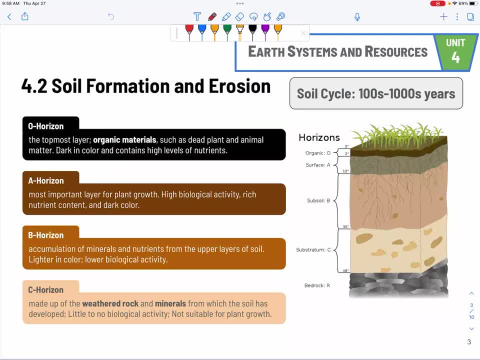 about soil. yeah, we talk about soil a lot in this course. we talk about soil in the section right here we talk about, in agriculture, deforestation. so it's very important to know all the horizons and the nature of the horizons, and on the left i have also included the color scales to help you understand. 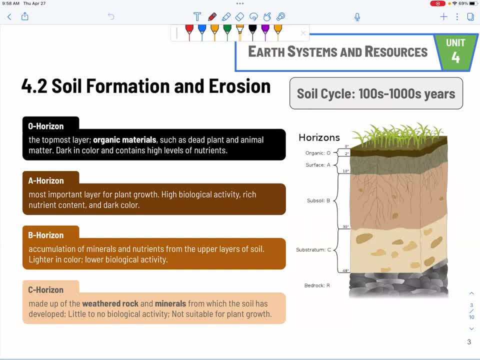 it better. uh, the old horizon is the one that's uh on top and that is, uh, the organic materials. uh, so that's why we call it. oh, because all the dead organic matters are going to stay there and be composed, so it's very rich in nutrients and that's also very dark because of all the dead organic matter that's. 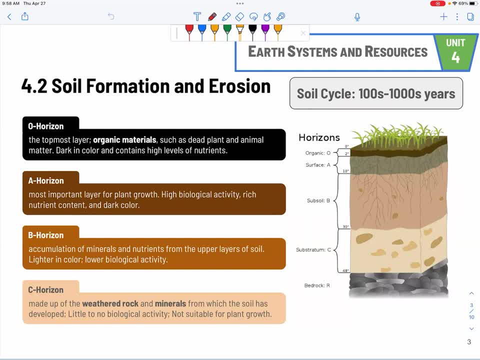 being oxidized by the bacteria, and then we have the a horizon. a horizon would be the one right below the a horizon, i mean the o horizon. you will see a lot of roots over there, okay, and a lot of organic activities there as well. rich nutrient level, because the nutrients from the o horizon 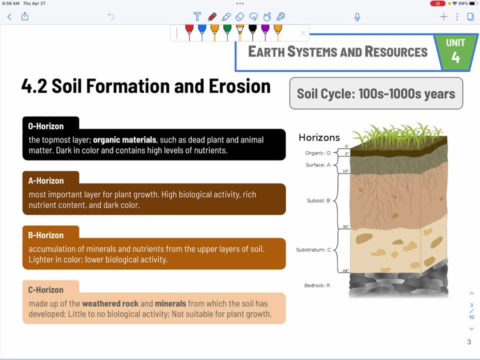 will just leach towards the uh. the a horizon, okay, so it's very dark, uh, and compared to your b horizon it's gonna be much darker, uh, because b horizons they don't really receive that much of a nutrient, so they don't look as dark as oh or the a horizons, uh. so they have some minerals, some nutrients, but not a lot. 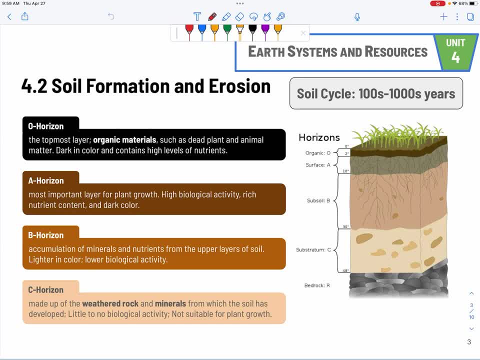 okay and you don't see a whole. i mean, you see some of the, some of the roots. maybe for trees they may go past the a horizon. of course they're going to dig deep, but not like a lot, okay. sea horizon would be the- uh, the mineral, the, the weathered rock, so you can see. 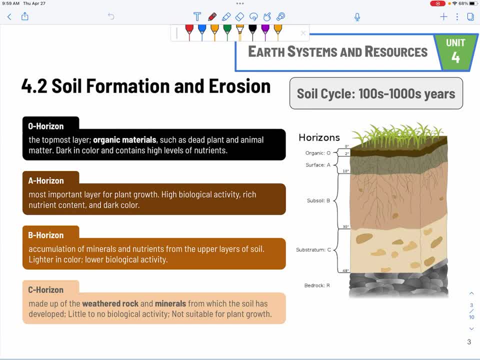 the big chunks, uh, of the rocks, okay, and the all layer is just the all horizon. it's just a bedrock, okay. look how we set about the primary succession. just bare rocks takes a long time in the soil cycle. it's really long. we're talking about hundreds to dozens of years. 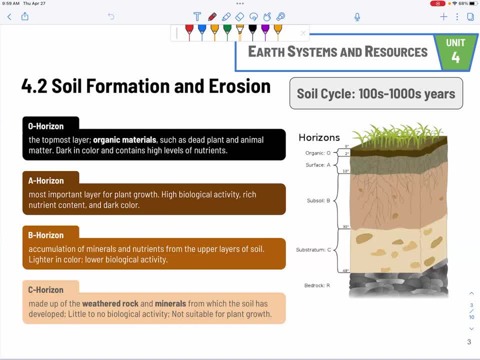 okay, uh, in order to uh, to, to form the soil and then the recycle the soil. okay, and that's all i want people to know on that as well, here why we care about soil erosion, because if the soil it hurts, it's going to take a long time to. 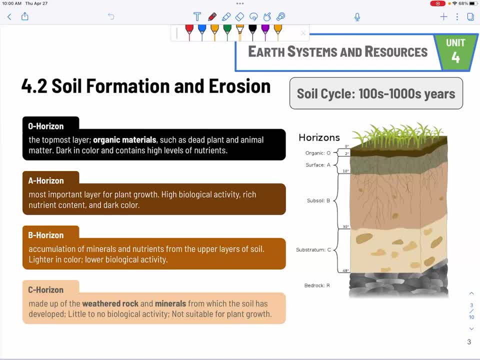 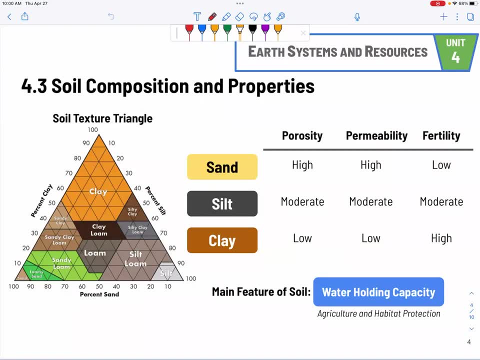 naturally recover it. okay. so make sure you know all these horizons, the location and also the uh, the features of each horizon. 4.3 continue to be about soil. it's about the soil texture, soil composition. we have three major types of soil. we have sand, silt and clay. all right, sand. 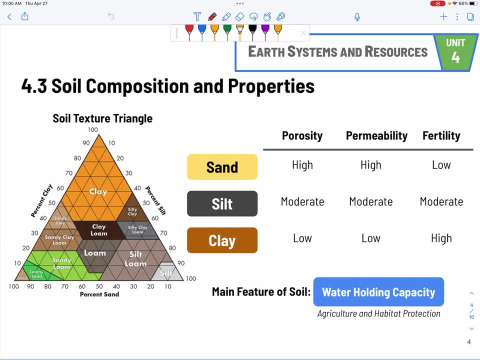 it's. uh, i think everybody has some experience with sand. they're coarse, uh, and you don't want to use sand to hold water because the water is going to seep through the cracks between the sand particles. uh, silt is somewhere in the middle between sand and clay and clay. it's very sticky. 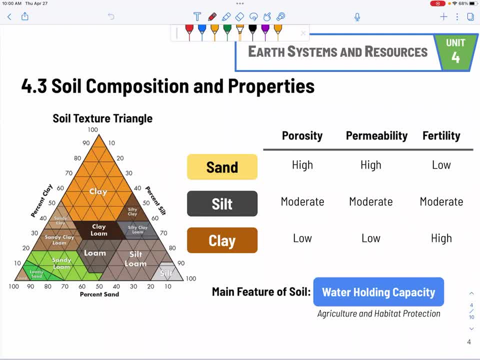 uh, very uh, not uh, permeable, okay, uh, in terms of uh water, um, uh flow, so uh. so, if you want to uh, we will use clay later on. we talk about, we talk about the landfill. okay, we want to protect the? uh landfill, we want to actually protect the underground water sources from the landfill, so we use clay as a way to uh, to. 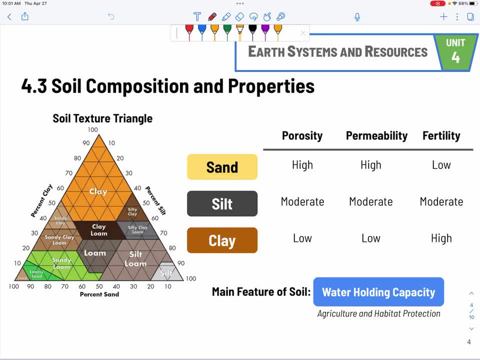 prevent any kind of water leakage or the leachate from going through the uh, the landfill. okay, uh, so you can take a look at the porosity, permeability and fertility. and clay is the has the highest fertility, the the the reason why they are so sticky, they're so, uh, impermeable. it's because of the stickiness due to. 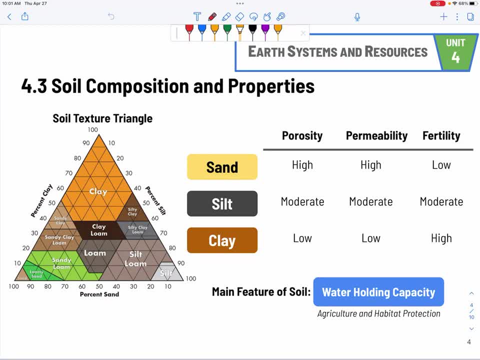 the ions, and the ions are the nutrition, uh, the nutrients, um uh, for the plants. so so clay it's very uh fertile, but uh, porosity and permeability, they're both very low, okay. so, main feature of soil: water holding capacity. and why we care about the water holding capacity is because we often 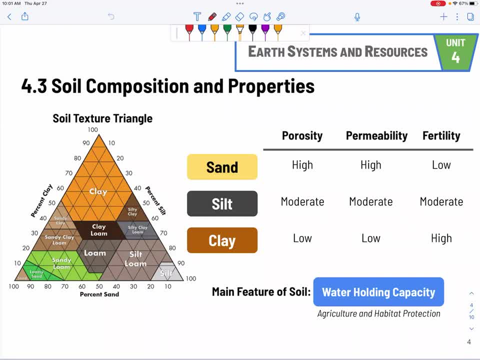 talk about wetlands and the asteroids and and a lot of deposits there, and the deposits are usually fine particles that would form clay and uh, and if they're able to absorb a large amount of water, then it's a good buffer to protect us from storm damages or the storm uh, wind erosion, um, so it's. 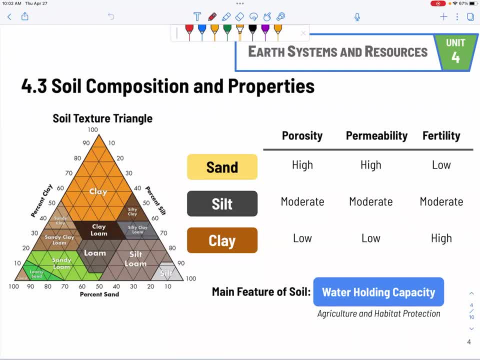 very important and uh, but as we're changing the land use, uh, these uh soil particles are being removed or they're not getting as many uh well, for example, clay particles or small sediments- as they used to be. so that's another reason why we care about the uh soil uh properties. all right, let's switch gear. 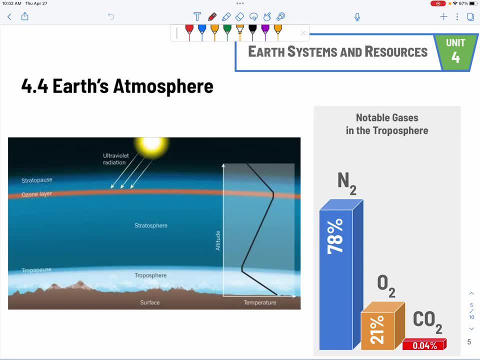 to talk about the air, the atmosphere. okay, the air and atmosphere. uh, one thing that everybody should know is the composition. if you receive a question about a composition, that's a guarantee that that's a gimme. okay, so it's a gift. okay, make sure you say thank you. so the highest amount of nitrogen. 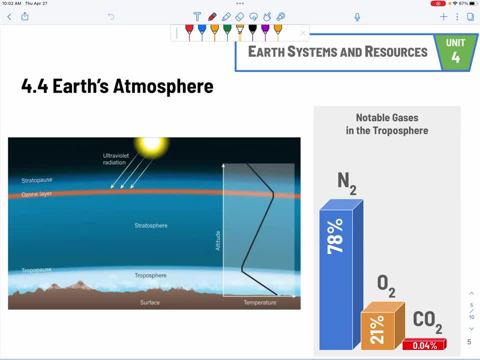 is the amount of nitrogen that's in the soil. okay, so the highest amount of nitrogen is the amount of nitrogen that's in the atmosphere, and it is the atmosphere. is this a major sink of nitrogen? 78 percent, uh, o2, 21 percent and uh co2- although we talk about co2 a lot, okay, in this course, uh, it is. 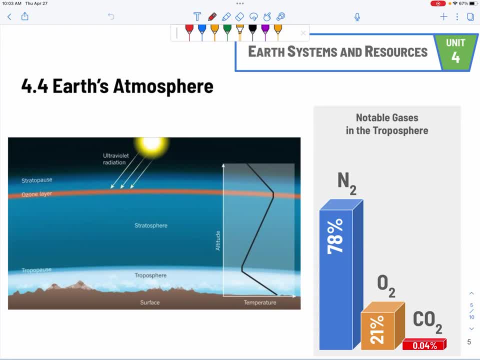 not like a huge percentage, it's 0.04 percent. now i just want to make one, uh, one major point right here, and people would think: well, if it's not that that big of a percentage, why do we care so much about it? well, that's exactly the point, because it's not that big of a percentage, it's not that big of a. 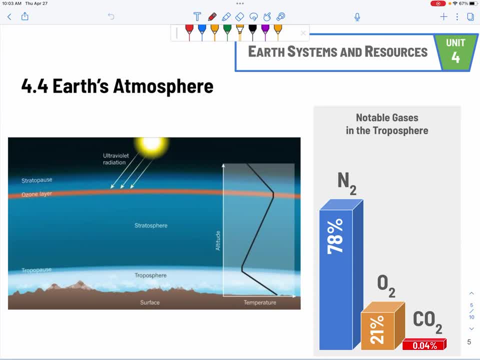 it's not a huge percentage, and yet it can cause such an impact. that's something right, that's something okay. so that's why we care about co2 and also methane. okay, since we are talking about carbon, uh, the atmosphere, uh, the most important two layers would be the troposphere and the 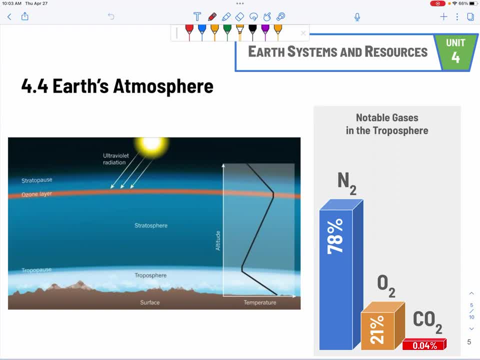 stratosphere. the troposphere is where we, where we interact with the gases. we interact with the gases, uh, in the atmosphere. now, the ground layer is where we see the weather. uh, the stratosphere is where we see the ozone layer, which protects us from uh, uvb and uvc. okay, so we have quite a few uh. 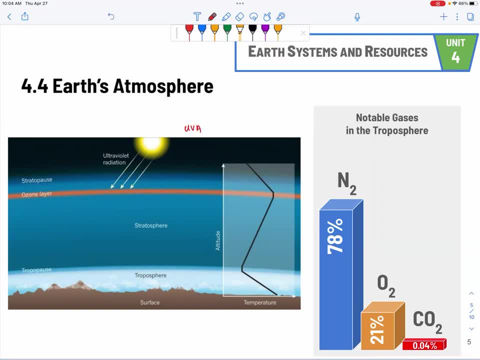 kinds of uv, uh, radiation, uva, uvb and uvc. a can pass through b, some could, some couldn't. uh, and uvc just stops right there, okay, so, um, so, therefore, it's uh, it's a very powerful thing uh that we have, and we're going to talk about that in a little bit, but before we do that, let's. 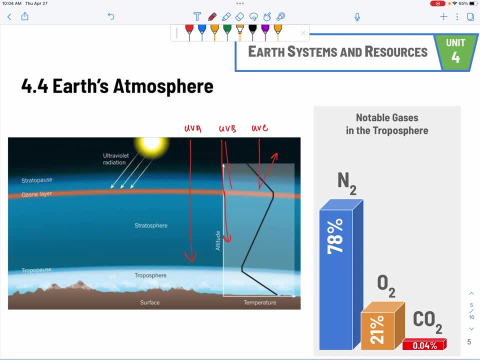 talk about the atmosphere. we're thankful for the existence of the ozone layer and if you know where this course is going. at the end of the unit nine, we also talked about the ozone depletion because, uh, something, it's hurting our ozone, so that's a problem. so making sure that you know. 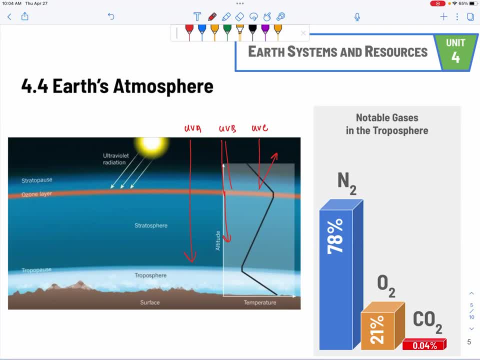 uh, the, the population, i mean the composition of the atmosphere, the layers. uh, there are some layers above it, the mesosphere and the thermosphere. don't usually see them, but, uh sure, why not? okay, now that's one more thing i want to highlight here, and that is the little temperature. 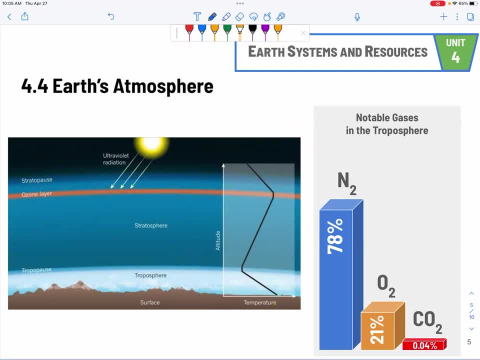 graph over here. okay, the temperature graph now. um, the reason i want to go over this is because the temperature does decrease as you climb higher, right, but because of the ozone, it actually increases again as you climb higher, and this is a huge, huge concept that i want to go over here. 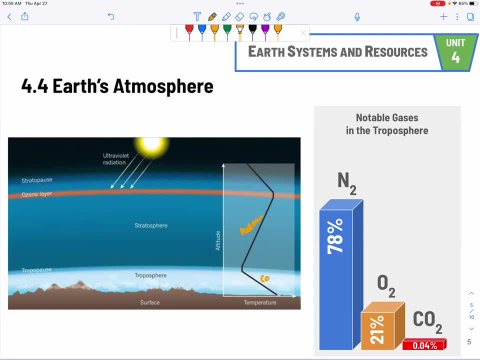 because it is warm above and a little bit cooler, okay, down below. it creates something called an inversion, okay, because, uh, the warm gas is less dense and that serves as a little lid, okay, to block the gas from escaping from this trouble. uh, triple sphere. now, this is also huge, because if you limit us with science, you know. 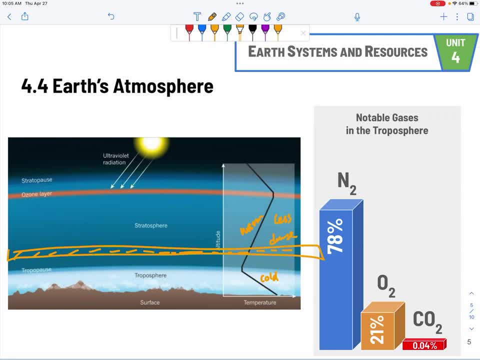 about diffusion, right. gas is moving from high concentration to low concentration, so the gases that we are breathing in right now, as we speak, should diffuse out of earth to space. technically right, but how come we can still breathe? it's because of this inversion, it's because of this lid, all right, because of the 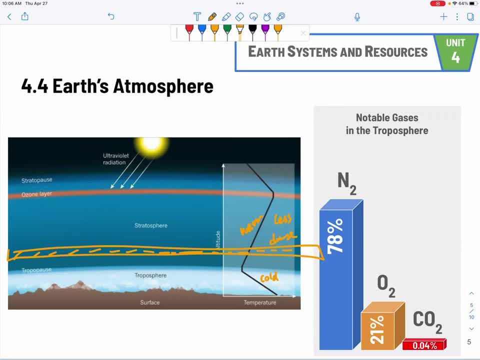 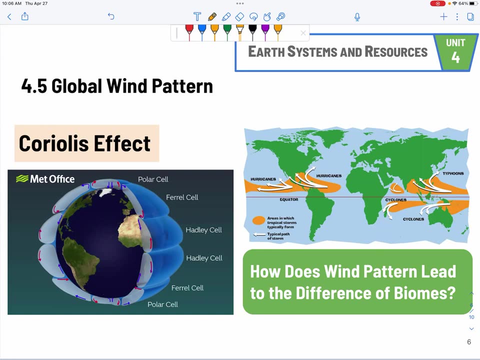 warmer air right above this troposphere. that covers it. if you understand this then it would help you understand, uh, air pollution stuff later on. okay, in this course, all right, uh, global wind pattern. global wind pattern, it's about, uh, the wind blowing. uh, now, without the earth's rotation, the wind would just go straight, okay, but with the earth's rotation, the. 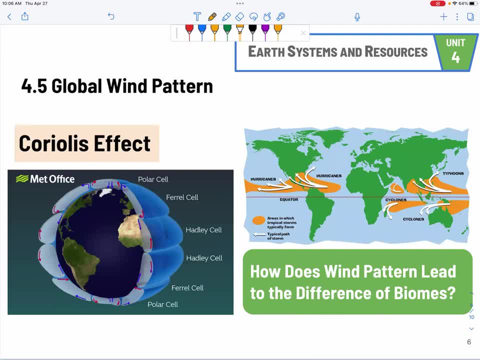 wind, the air particles, the wind, they are going in circulation. so the, uh, the cells that we see over here, the headly cells, uh, in the north and the south hemisphere, the ferro cells, polar cells, like they are only cells because of there are three separate cells, because of the earth's rotation. 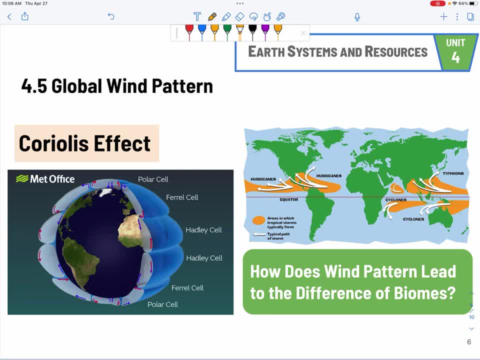 if there are no such cell. okay, if there are no such, uh, i mean there's no such earth rotation. there will be one big cell in the northern hemisphere and then one big cell in the southern hemisphere, that's all okay. uh, so the reason, so the rotation, here it's called the. 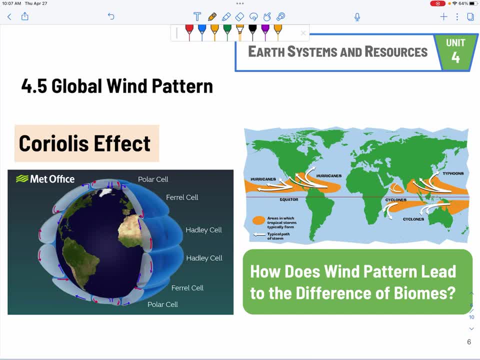 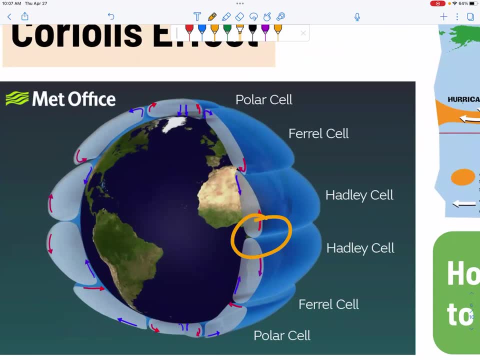 coriolis effect, and this is where we see the trade winds and the uh and, of course, these cells on the left diagram, uh, like the increasing part right here. well, that's because it's hot, okay, that's because it's hot. and then the air is going to sink at this region at about 30 degrees north and south. 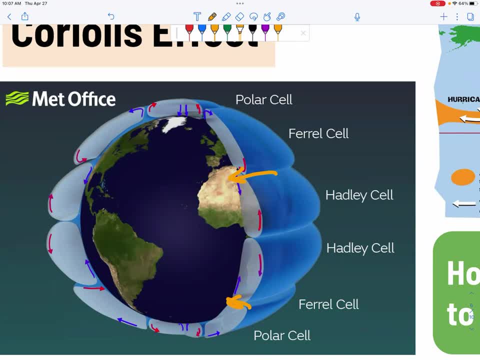 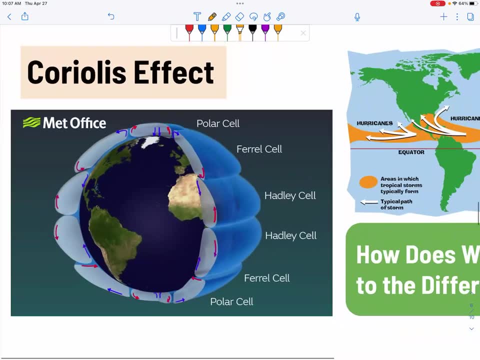 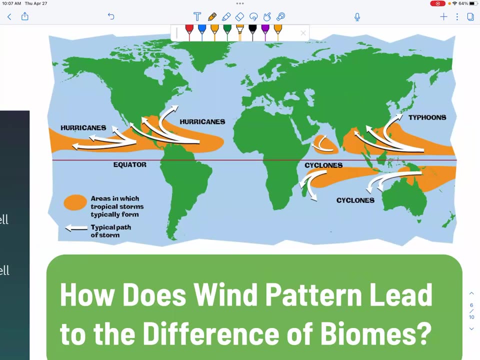 latitude and that it's going to cause the formation of the deserts, because the air is dry and the pressure is high and there's no, not much of a precipitation in those uh, latitudes, okay and uh, and the reason why these hurricanes or typhoons or cyclones are always moving in such direction? 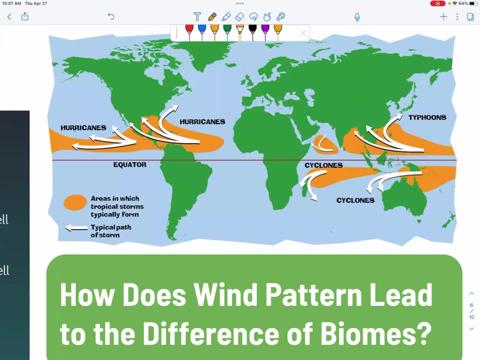 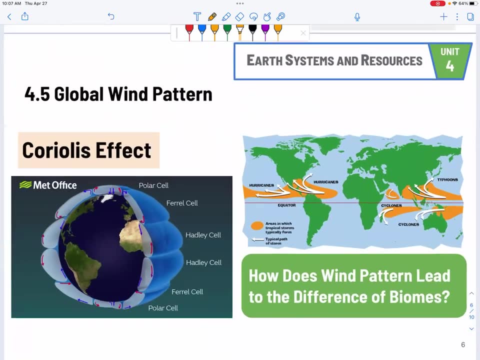 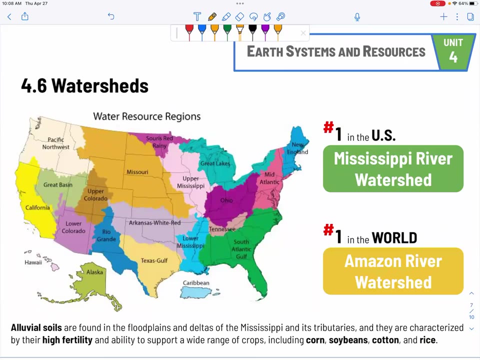 is because of trade winds. okay, the westerlies and the easterlies. okay, we call them trade winds because, well, you know, as the name suggests, they're for trading. okay, so, uh, so it's very impactful back in the days. watersheds: major thing about watersheds is the. the idea of watershed is like a bowl. okay, it's. 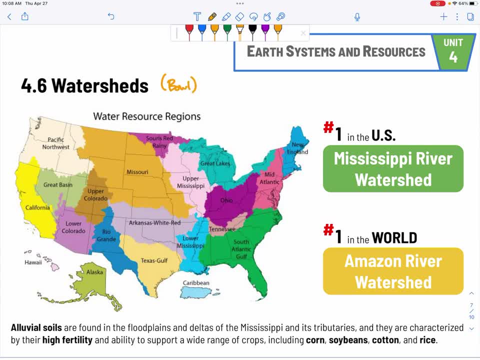 like a bowl that collects all the rain in that region and the number one watershed it's going to be the mississippi river watershed, which covers all all the way here, okay, all the way here, okay. so a lot of states are being covered, and um, and then, uh well, 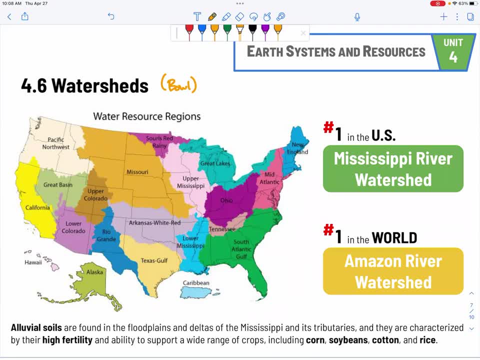 why do we care about watersheds? because, well, first, water supply, okay, uh, the, the, the snowfall and the winter, the rain, the springtime, summertime, will we have enough water for agriculture, for drinking? that's one major thing that we care about watersheds. and then the other thing, it's: 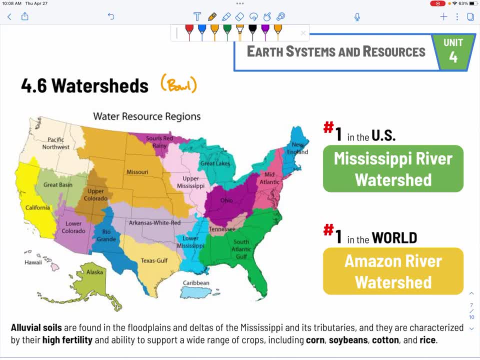 about pollution. uh, anywhere that's polluting the watershed. inside the watershed, it's going to affect the water sources downstream, so that's why we care about the watershed here. okay, uh, that's a mississippi river watershed. it's number one in the us, number one in the world. 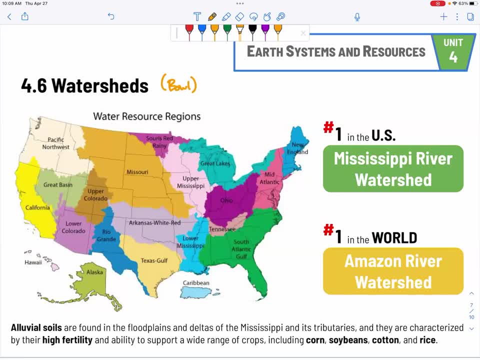 is the amazon river watershed. okay, uh so, uh so, at the end of the watershed, uh, it's uh where the flood, where you find the flood plains, uh, so, near the uh mouth of the mississippi river in the, in the state of louisiana in new orleans, uh, where you will find a lot of alluvial soils. they are very 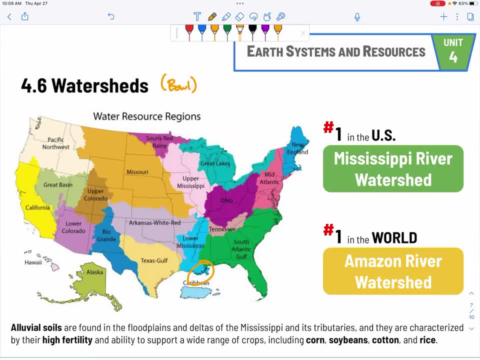 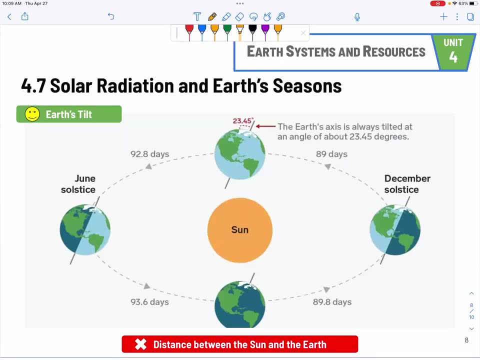 nutritious, they're high in fertility, they're very nutritious, they're high in fertility, and then we can use it to uh to grow a lot of crops, such as the one down below, corn, soybeans, cotton and rice. okay, all right number is 4.7. it's a solar radiation and seasons. simple thing, but a 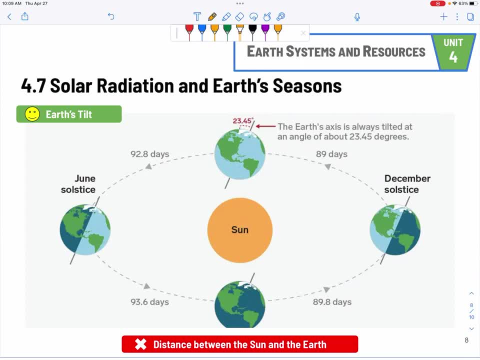 lot of people. they get the misconception. the reason why we have the season is because of the tilt, not because of the distance. but why would people think about distances? because of the diagram right here, see, like right here it seems like a short distance, but then, uh, but then if you look at the distance, 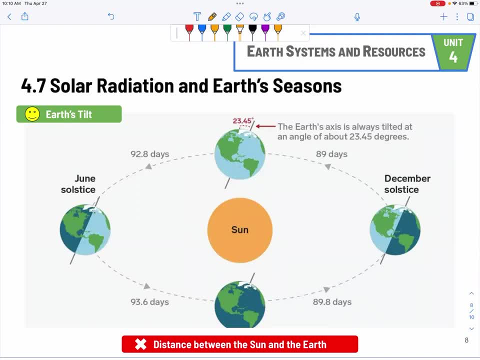 right here. it seems long. so people think about: oh, it's probably the distance, right? nope, earth, uh, although it's not a perfect circle, but it's pretty darn close to a circle. so the distances between the earth and the science wall is constant. it is a tilt, the 23.5 degree tilt that led to the 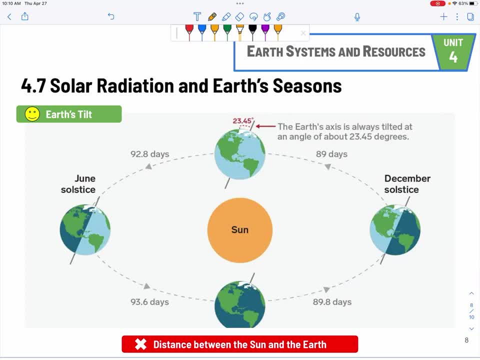 formation, the, the appearance of different seasons of this planet. uh, equator, of course you expect to be long, and then northern hemisphere, okay. um, you know, summertime, wintertime, at the months that most people would experience, you know, june, july would be the summer months and then the winter months will be december, january. okay, 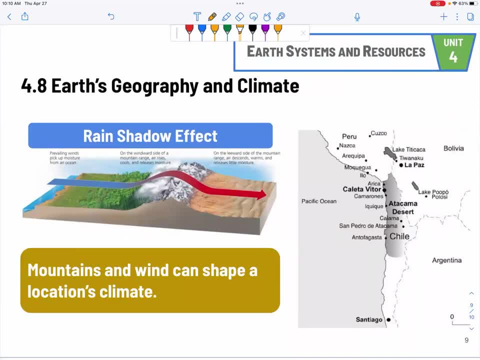 uh. next one, it's the, uh, the earth's geography and climate. okay, so a couple of things right here: rain, shadow effect, mountains can shape climate. okay, mountains can shape climates. if you live in the states, then you know how we have, uh the. in the west coast we have the sierra, sierra nevada, uh. 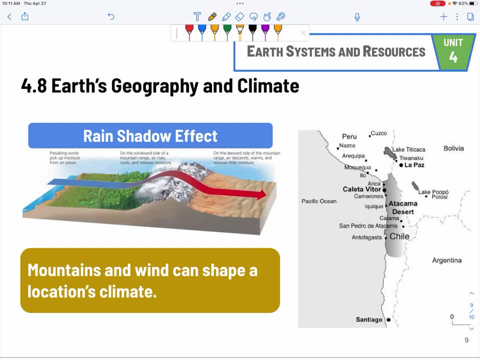 mountain range and then on the west side, in the california side, where you have a lot of vegetations, you see the redwood trees. but then, after like beyond the mountain ranges, which is on the east side of the mountain ranges, we have nevada, arizona. we are like bone dry deserts. okay. 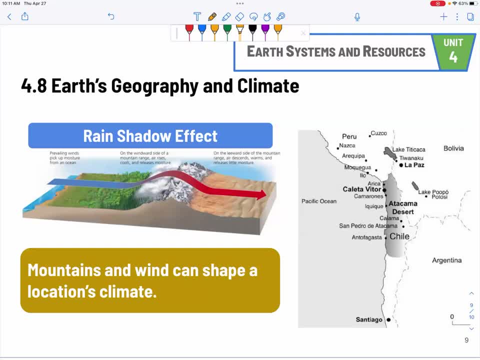 so all and the reason, the explanation it's because of the range of the ocean- is because of the, uh, the, the shadow effect. okay, uh and uh, the. the map that i show you on the right it's a map of chile, and the reason i want to show it is because, uh, it's right. next, 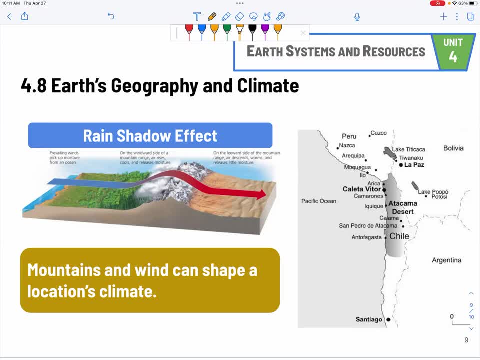 to the ocean. the entire country is right next to the ocean but yet we can have a desert next to the ocean is because of the wind pattern. wind pattern can change a place climate. i think that's very reasonable, right and uh. and even it's right next to the ocean, we could still have a desert. so 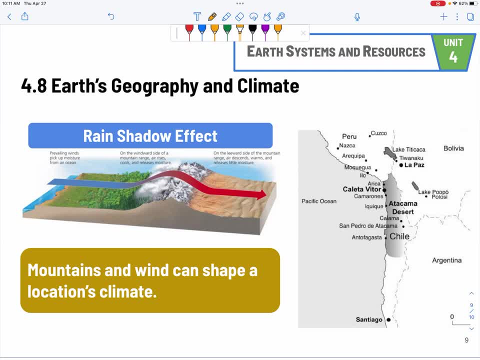 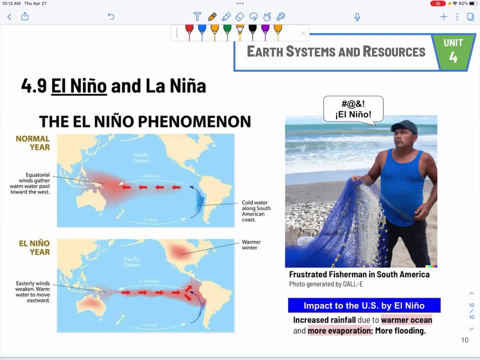 uh, so this is why, um, uh, geography is such an amazing topic, okay, and last one is el nino, and, okay, i'm gonna focus on el nino. so the opposite would be true for a lot. now i i have the- uh, the fisherman right here on the right. um, it's ai generated, it's an angry. 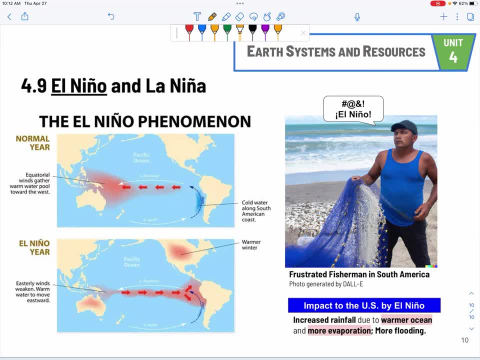 fisherman, because you can see here. and why do we call it el nino? because it's a curse. actually, it's uh for jesus, uh, when do we call jesus out? it's when we are angry, right, jesus? so, uh, so, because the wind stops blowing in the um south america uh region, or the central america. 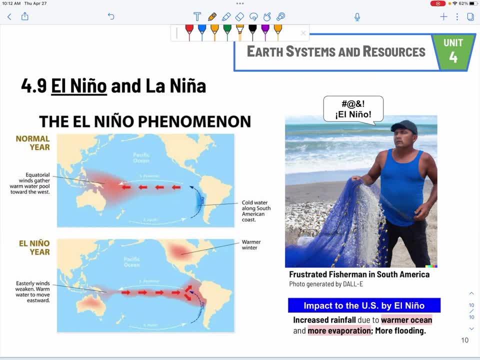 region. that's why the fishermen, they are angry, frustrated. okay, there's no fish, uh, and of course we can go deeper, to the formation of the appearance of upwelling, which is how the wind blows the water off the coast and drawing the bottom water up. so, without the wind, as you can. 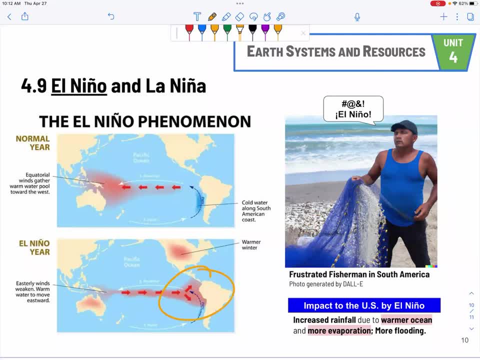 see from the bottom diagram right here: with thatцы the wind, the water gets warmer and there's no upwelling. and the fishermen? it's sad. now the fishermen could be sad, but in the us we are pretty happy because with el nino we tend to receive a.